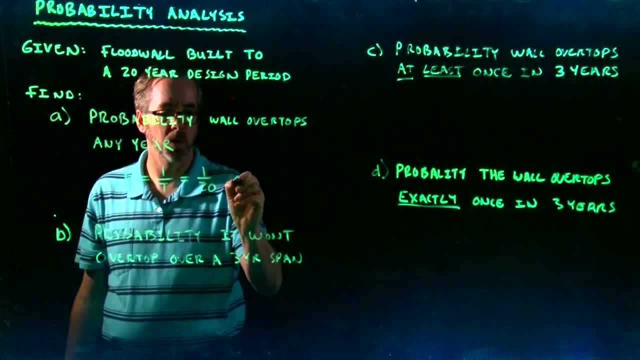 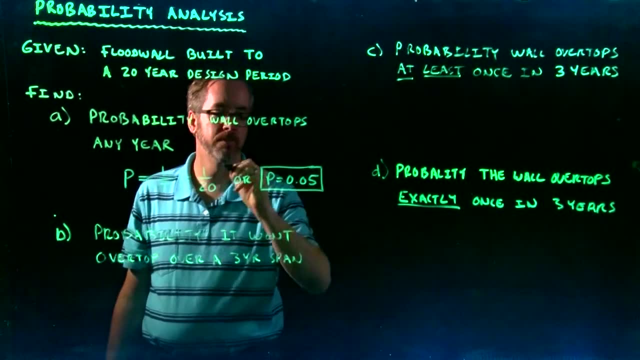 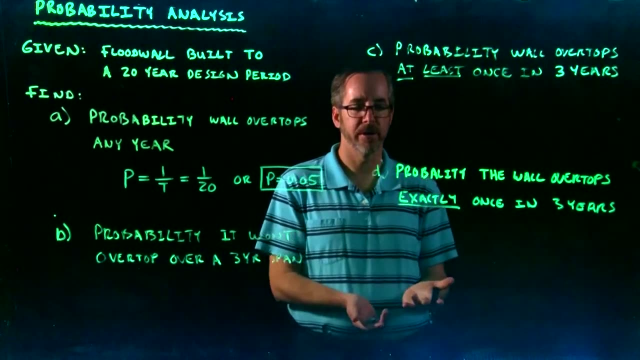 So in this case it's 1 over the 20 years, or the probability will be just 0.05, or 5%. Okay, Very straightforward. Now what's the probability that it won't overtop in a three-year period? 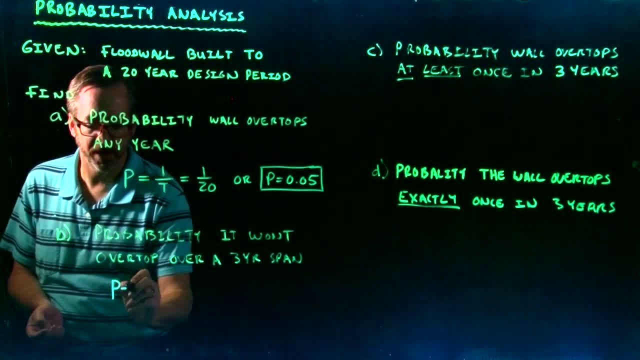 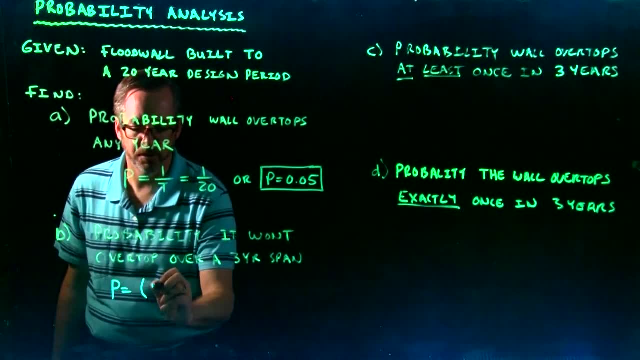 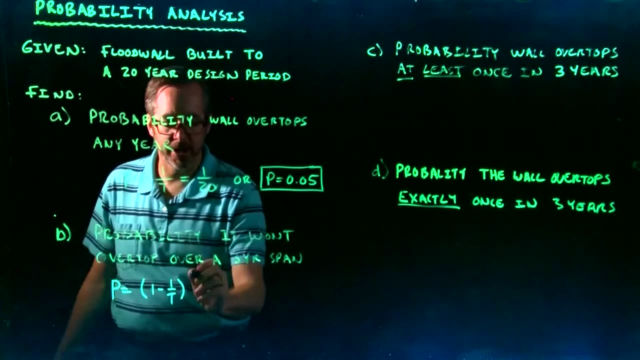 Well, if the probability that it overtops in one year in any given year is 1 over t, the probability of the first year it won't flood is 1 minus 1 over t. Okay, And likewise for the second year, the probability that it doesn't flood is 1 minus 1 over t. 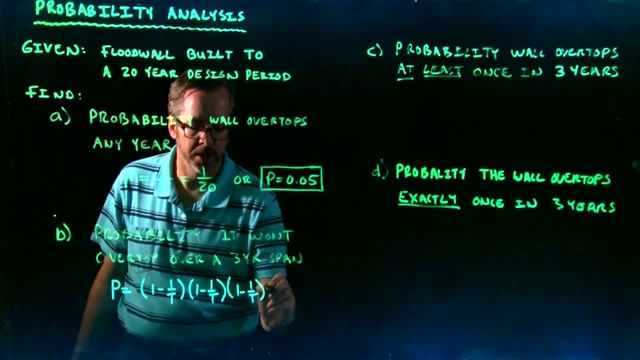 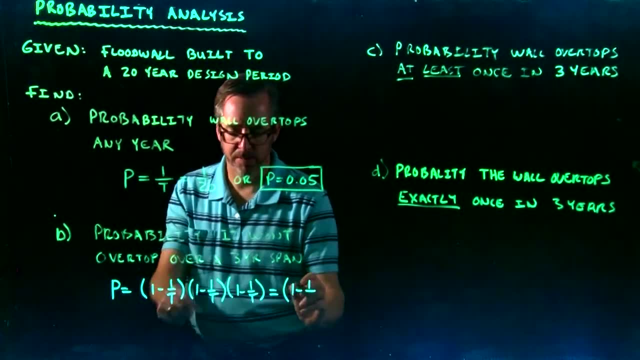 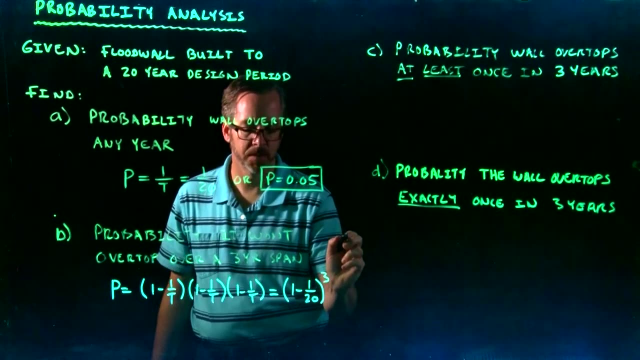 And then the third year: 1 minus 1 over t. Okay, That also could be written as just 1 minus 1 over the period, in this case 20 years. all that to the third right, Because we have three years. Okay, And that gives me a probability of 0.857, or roughly 86%. 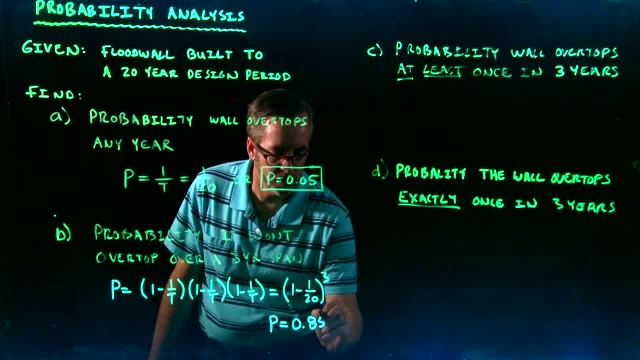 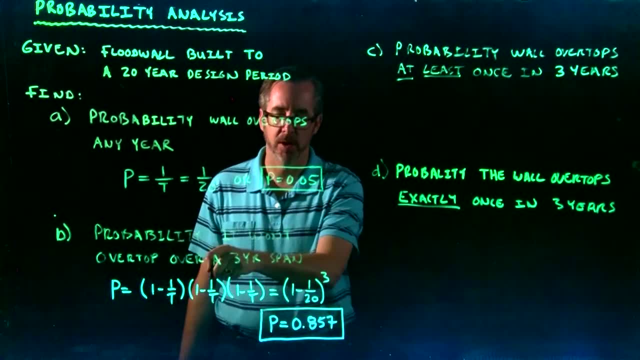 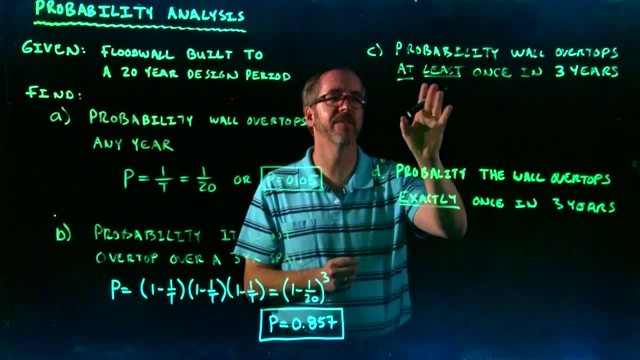 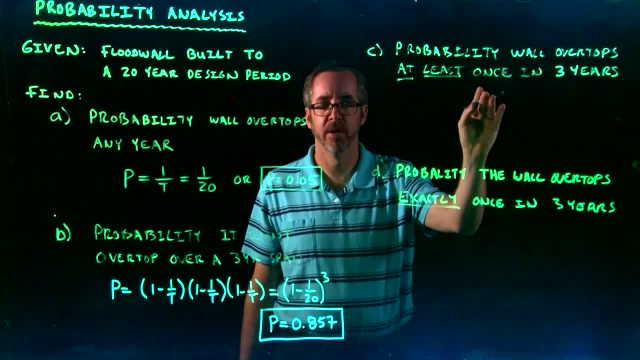 that three-year span. Now in part c we want to figure out, well, what's the probability that it's going to flood or overtop at least once, So it can flood more than once. It can flood one, two or three times in that three-year period. Okay, So for this we have to look. 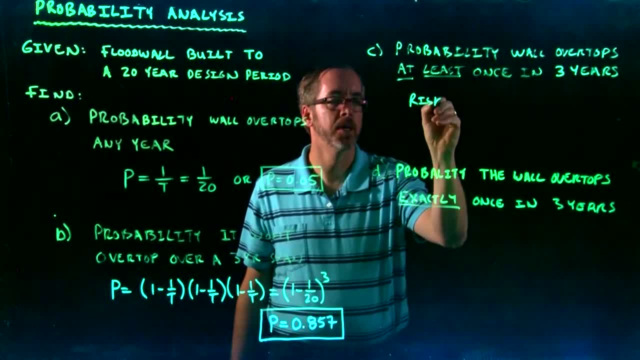 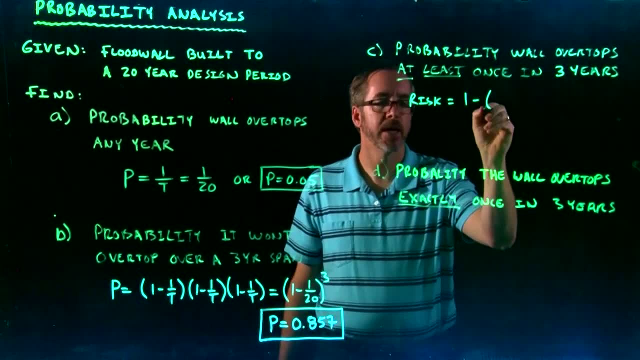 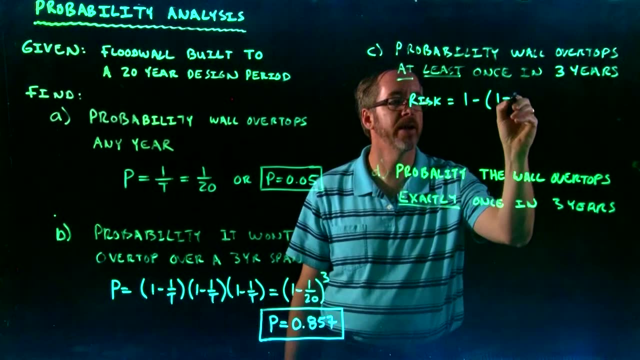 at the risk. The risk is literally 1 minus the probability of the event. So on this particular case it's going to be 1 minus, and then we have the probability that it will not flood in. a three-year period was 1 over- I'm sorry- 1 minus 1 over T. so this would 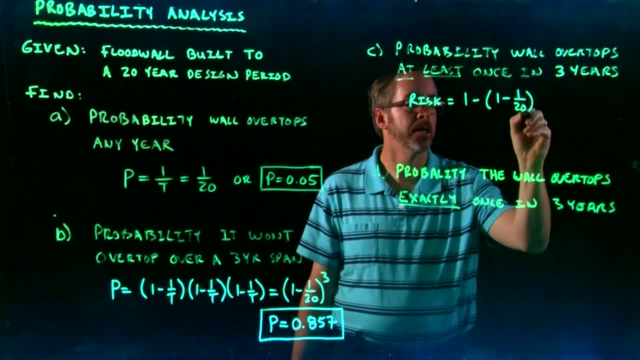 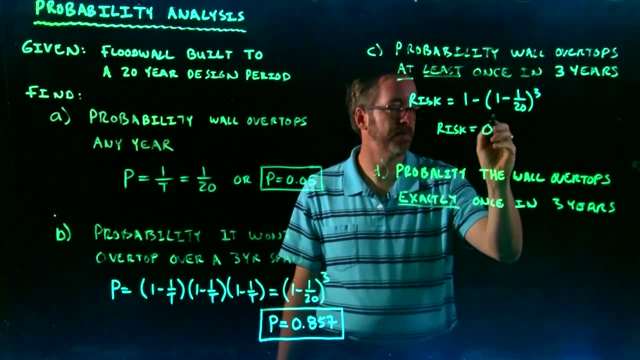 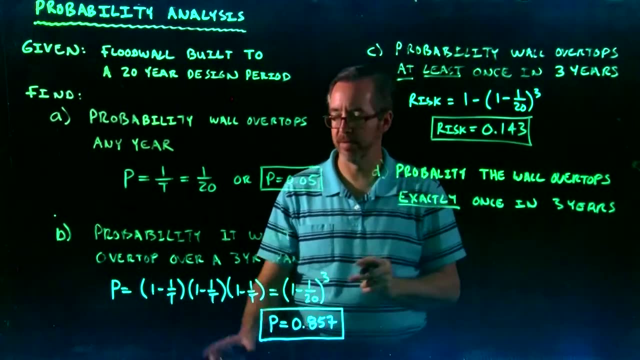 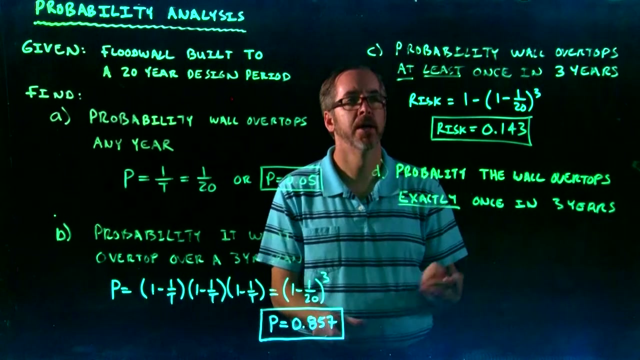 be 1 minus 1 over 20 to the third. okay, and this gives me a risk of point one, four, three. so what we're saying is is in Part B, if we're saying the probability that it will not overtop in a three-year period is 86% roughly the probability. 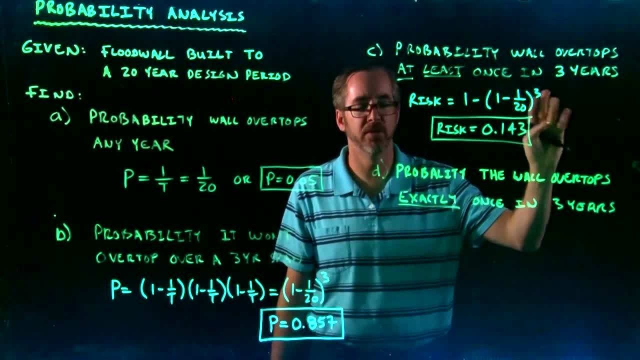 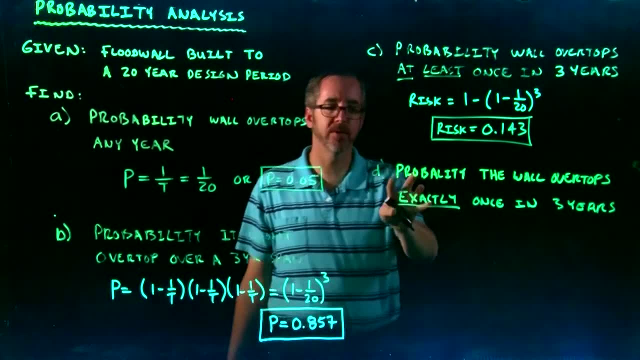 that it does overtop at least once. it could do one, two or three times in that three-year period would be roughly the 14%. okay, now what's the probability in Part D of that if flooding exactly one? so here was the probability that it at. 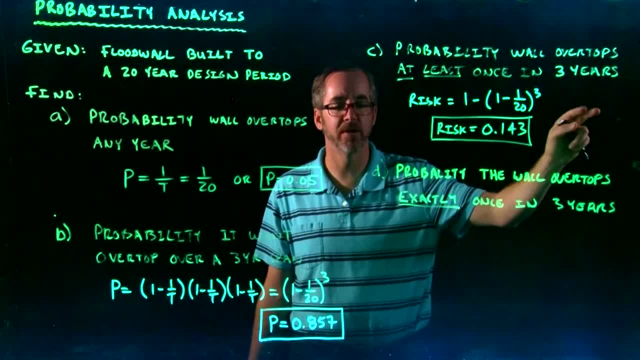 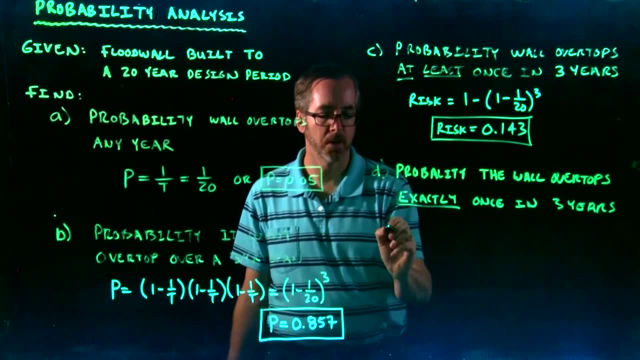 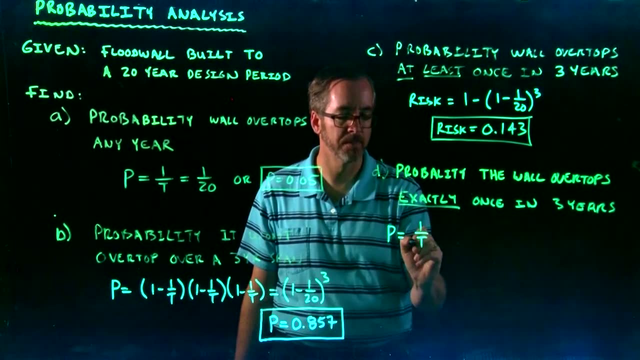 least floods one time in the three-year period and it does overtop at least once, but it could be one, two or three times. in this case, we want to know what the probability is of having it occur exactly once. okay, well, in a three-year period, let's say, for example, it occurs the first period, the first year, okay, so. 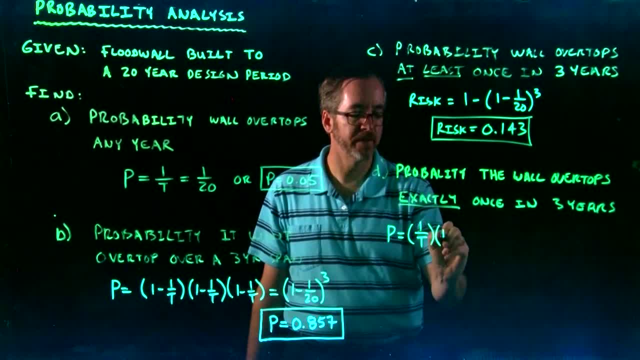 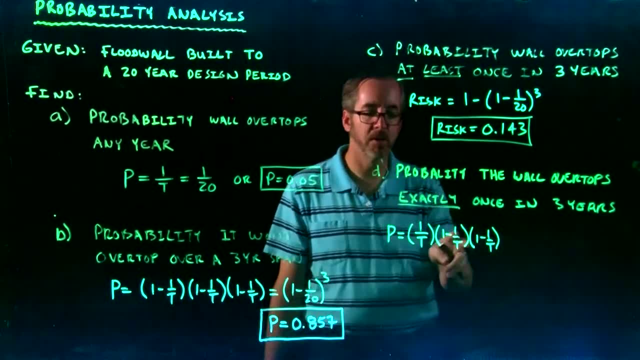 that would be the first year, but it doesn't occur for the second year and it doesn't occur for the third year. okay, so that's a scenario where we have the probability of it occurring the first year, but not the second or not the third. Well, what happens if it goes? 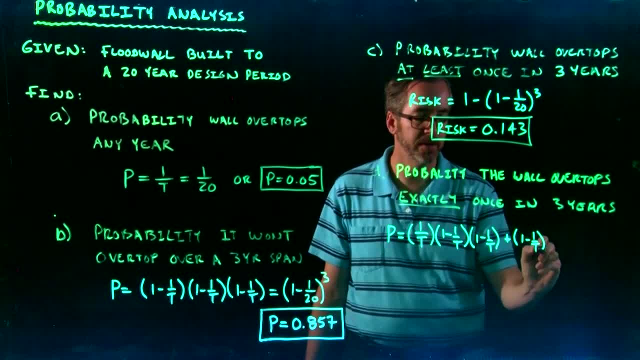 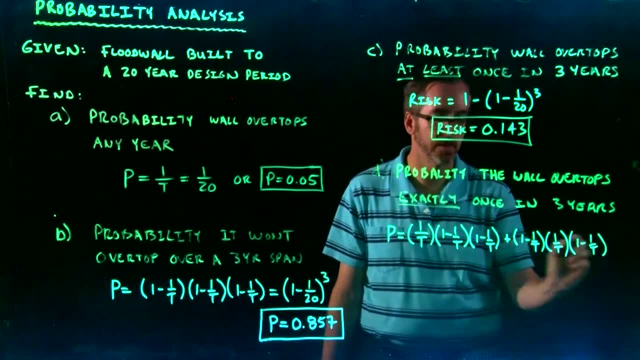 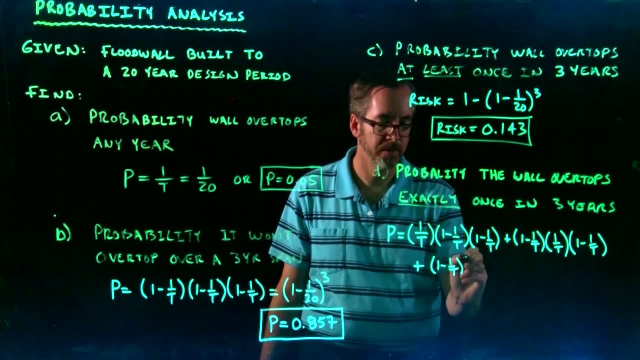 the second year. So the first year it doesn't, the second year it does, and the third year it doesn't. Okay, what about if it occurs the third year but not the other years? So year one doesn't occur, year two doesn't occur, year three it. 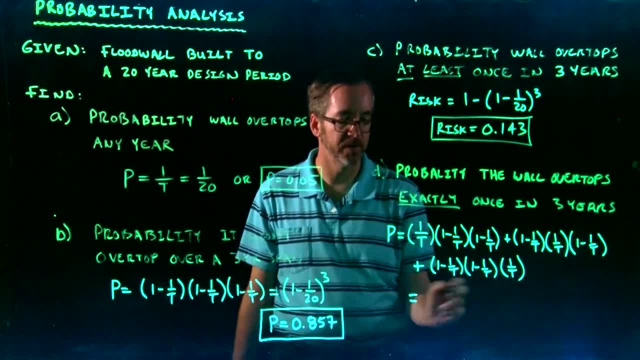 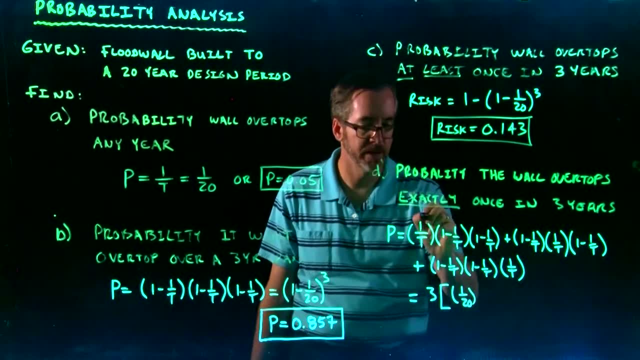 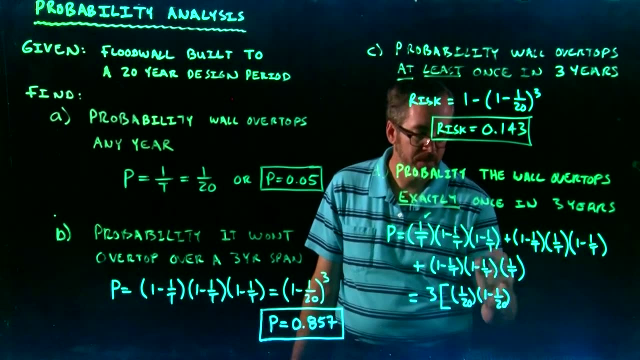 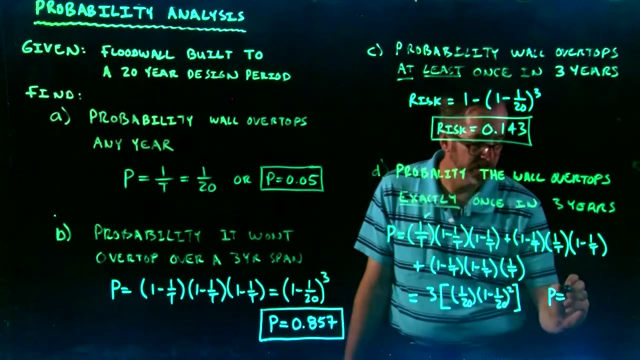 occurs. Okay, so all this reduces to essentially three times. you're gonna have the 1 over t term right from this piece, and then we're gonna have 1 minus 1 over t and this is squared. Okay, this probability comes out to be about point. 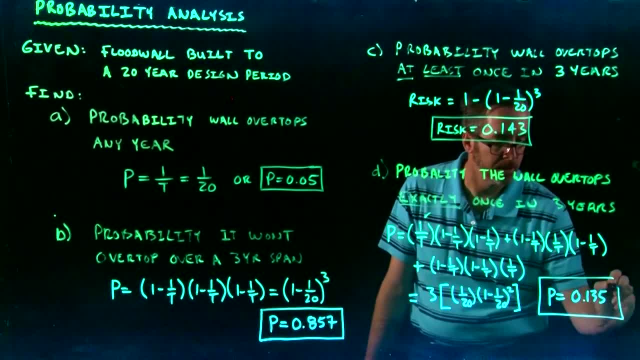 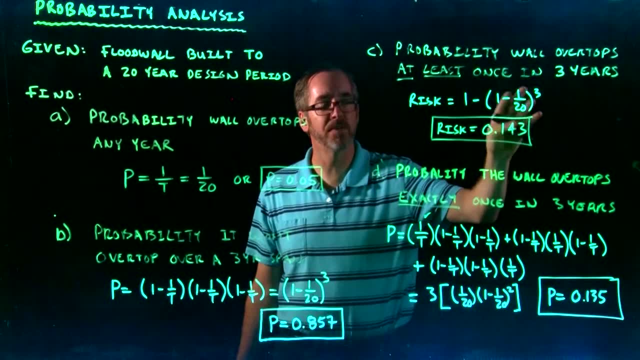 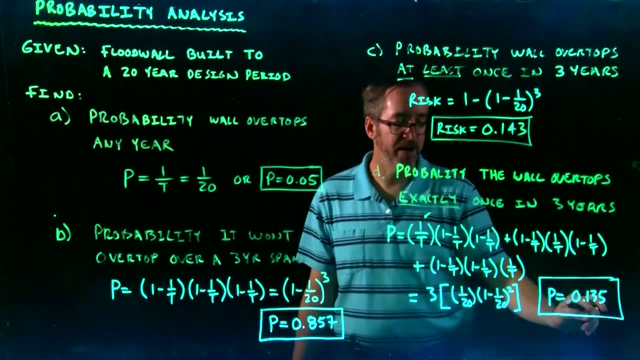 one, three, five or thirteen and a half percent. So what we're saying is is that there's a probability of it occurring at least once, but possibly two or three times in a three-year period of 14%. The probability that occurs is exactly just once is roughly thirteen and a half. 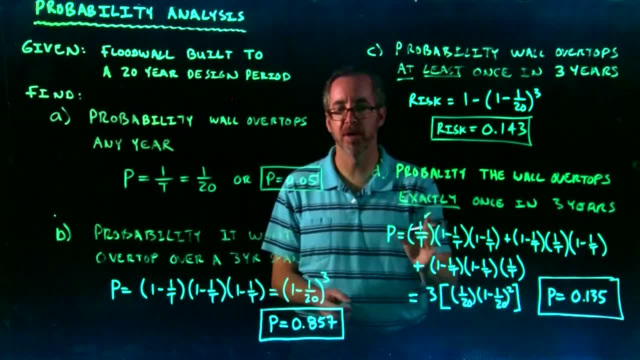 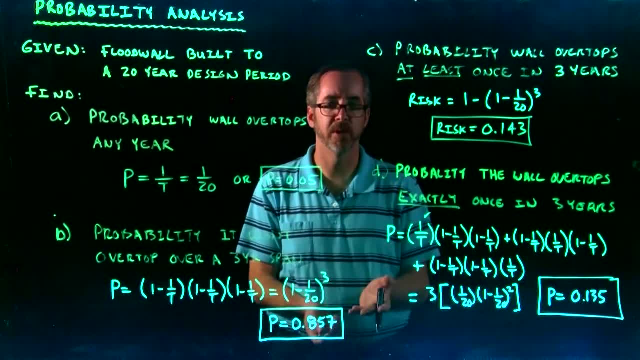 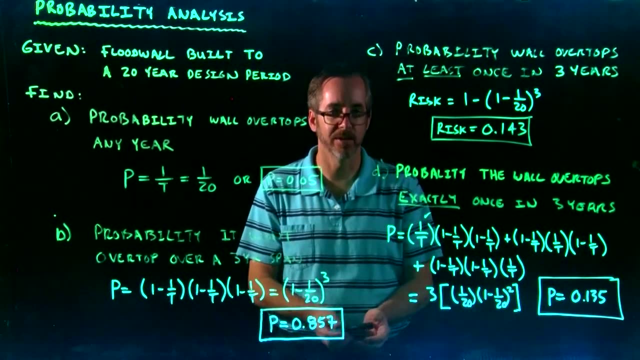 percent. So again, with this we've gone through and done an example in which we utilized probability analysis for the flood wall that was built, a twenty year period in order to determine its risk and their different, several, several probability factors. That concludes this example.